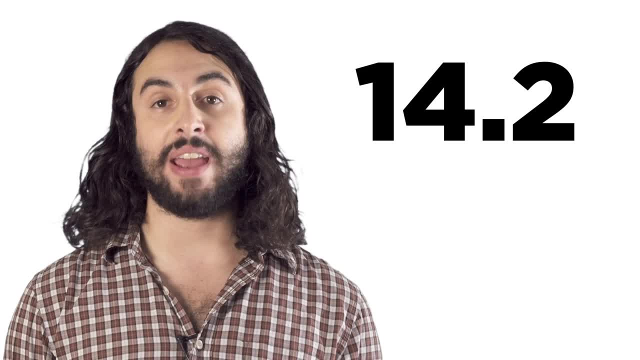 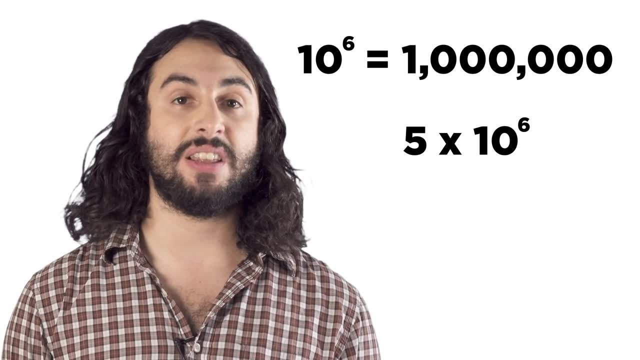 142.. We can get that by moving the decimal to the right twice 10 to the sixth, or a one with six zeros is a million. So 5 times 10 to the sixth is 5 million. We can get this by moving the decimal over six times, adding zeros if we need to. 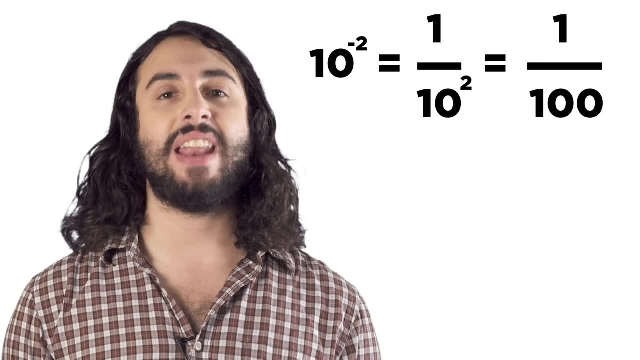 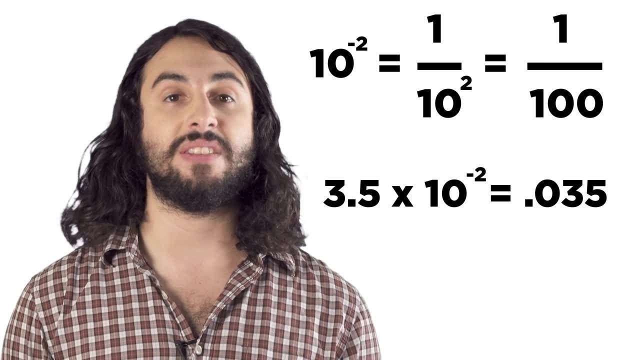 We can also discuss very tiny numbers this way: 10 to the negative second means 1 over 10 squared, or 1 one hundredth. So 3.5 times 10 to the negative 2 is 0.035.. We can get this by moving the decimal two places to the left, and 8 times 10 to the negative, 9 will be this number. 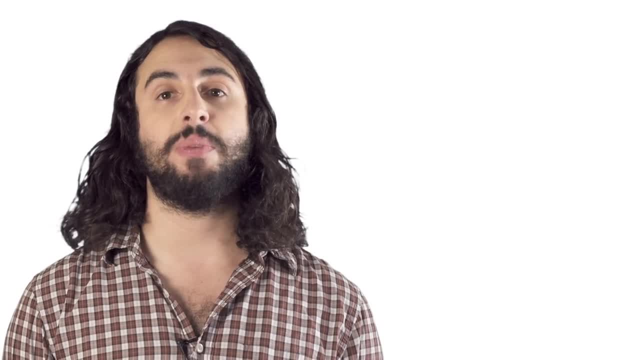 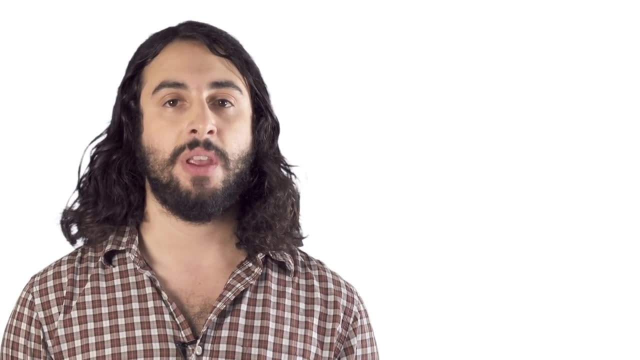 once we move the decimal nine times. This is useful because now we don't need inches and feet and miles, We can just use one unit and express values in scientific notation: For length we use meters, for time we use seconds and so forth. 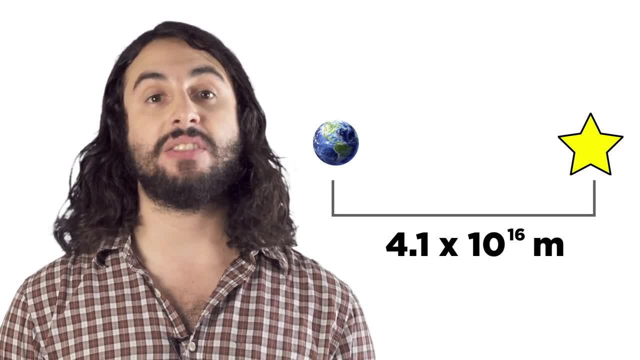 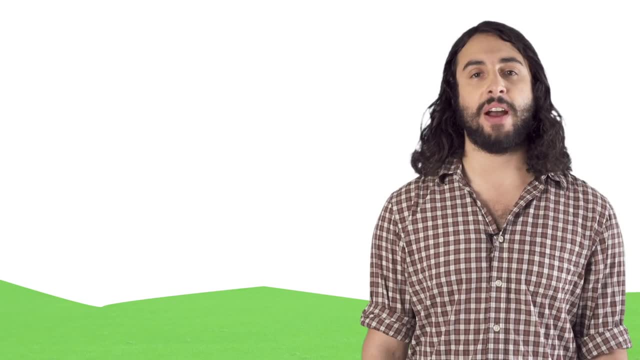 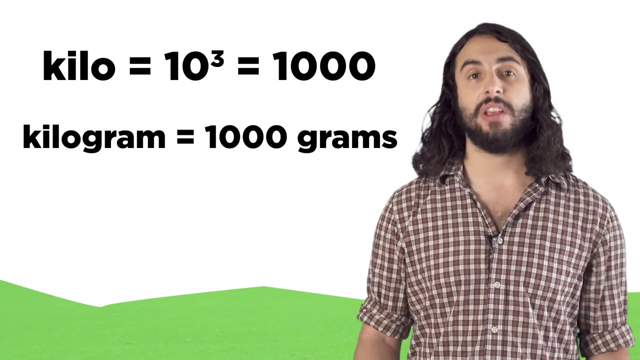 Now we can discuss the diameter of an atom and the distance to the nearest star in the same unit, meters. just with scientific notation, We can also use unit modifiers to symbolize different magnitudes. Kilo means 10 to the third, which is a thousand. So a kilogram is a thousand. 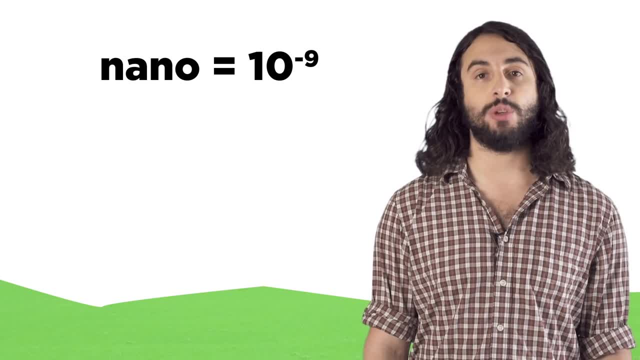 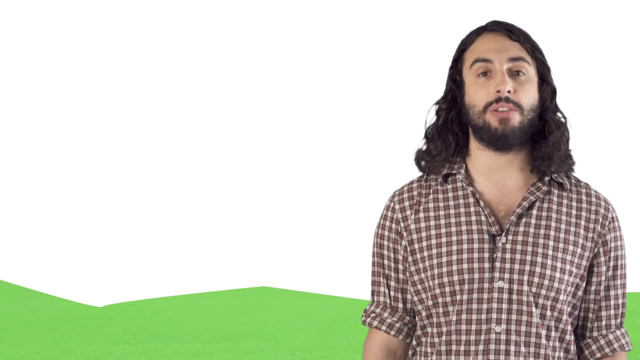 Nano is 10 to the negative 9,, which is 1- one-billionth. so a nanometer is this many meters. So we can express values with a word to indicate magnitude instead of a specific factor of 10.. Here are the different modifiers we use. 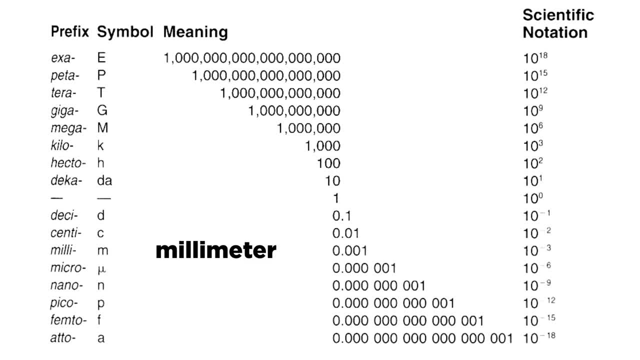 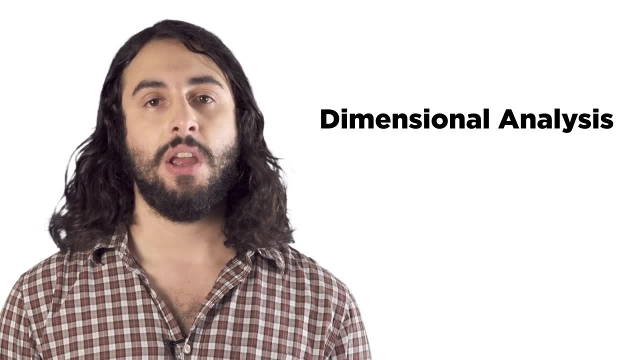 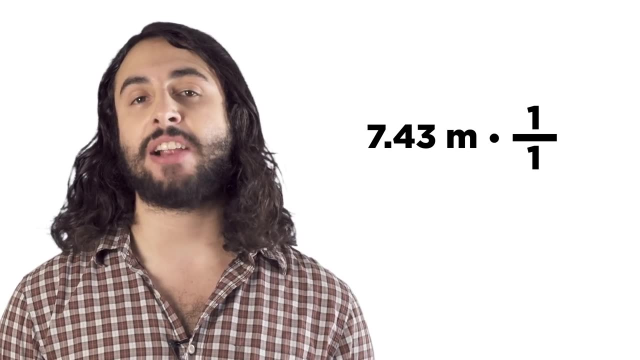 We can apply them to any unit and they will do the same thing. To convert between units we need to do dimensional analysis. Let's say we have a value in meters that we want to express in nanometers. We take the value we have and we multiply by a fraction that is equal to 1.. 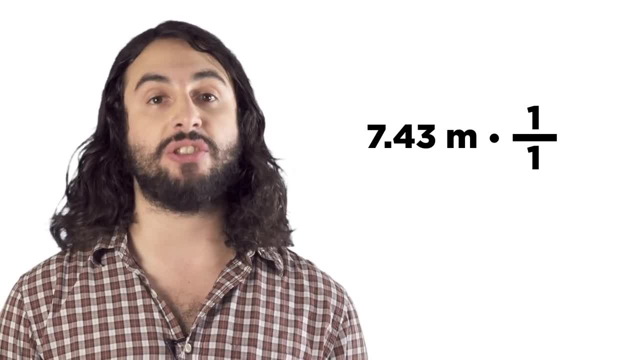 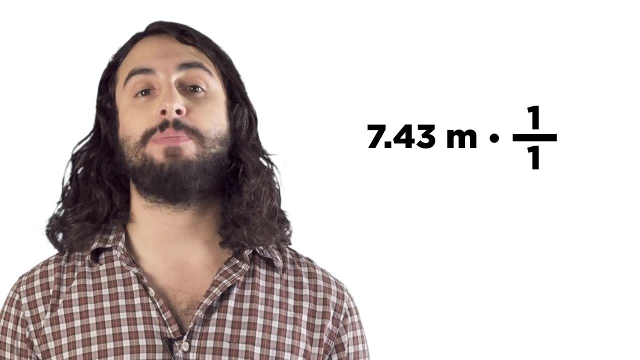 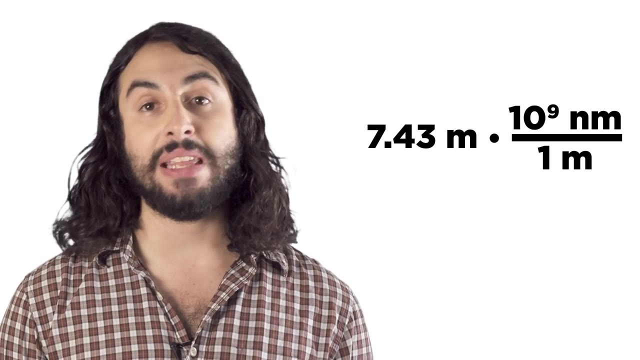 We do this because multiplying by 1 doesn't change the value, But we multiply by a version of 1 that changes the way the value is expressed. We do this by putting things on the top and bottom that are equal to each other, In this case, 10 to the 9 nanometers on the top and 1 meter on the bottom. 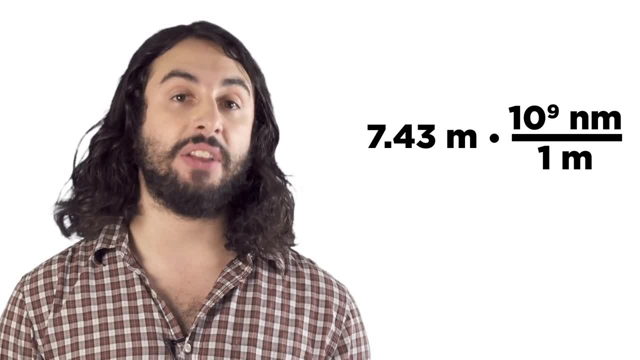 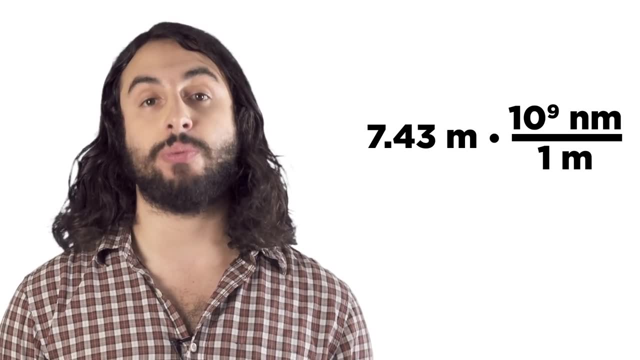 These are equal because if a nanometer is a billionth of a meter, then there are 1 billion of them in one unit. So, since these are equal, this fraction equals 1, but the meters cancel, just like an algebraic variable.